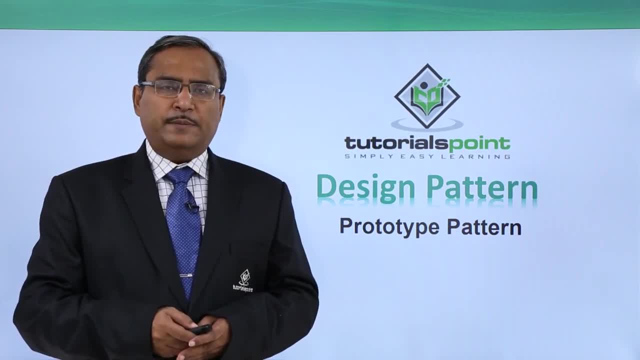 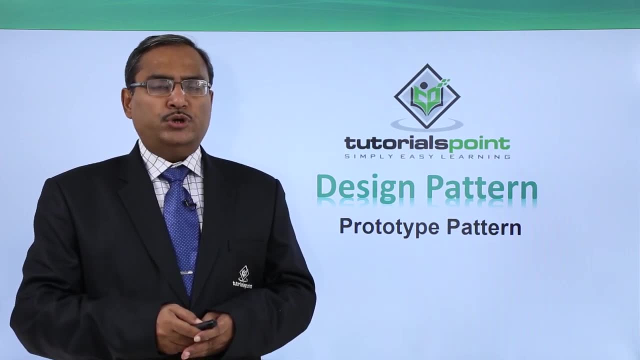 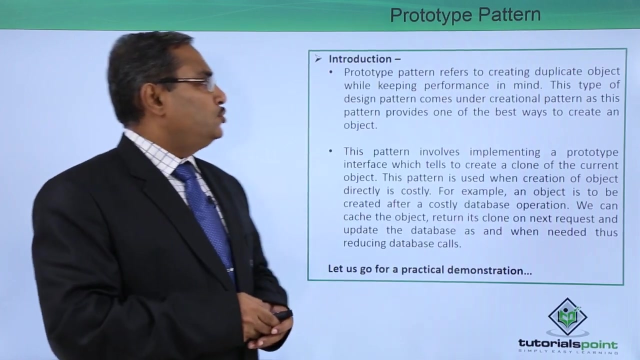 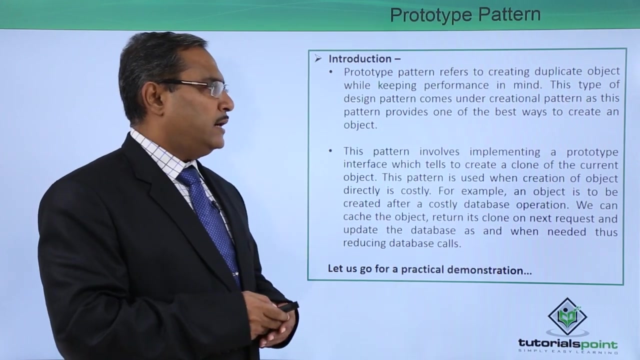 Prototype design pattern. This design pattern is also falling under the creational design pattern category. In case of prototype design pattern, we shall create a copy of one object, keeping the performance of the system in our mind. So prototype pattern refers to creating duplicate object while keeping the performance in mind. This type of design pattern comes under 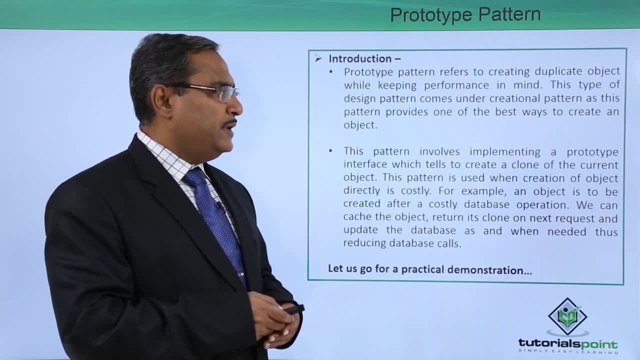 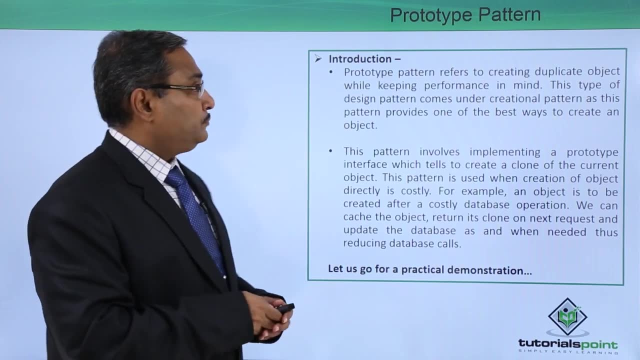 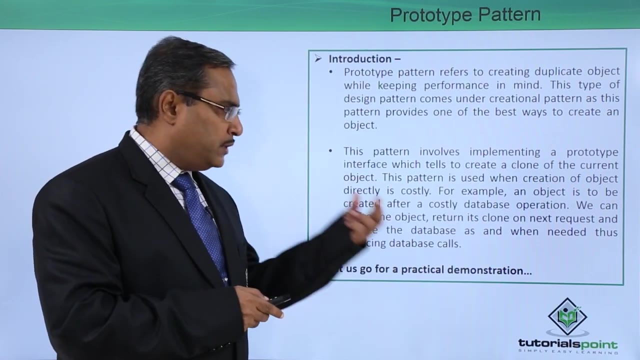 the creational pattern, as this pattern provides one of the best ways to create an object. Now, what is the basic theme behind this particular design pattern? In case of prototype design pattern involves implementing a prototype interface which tells to create a clone of the current object. So to create a clone that is, a copy of the current object. This 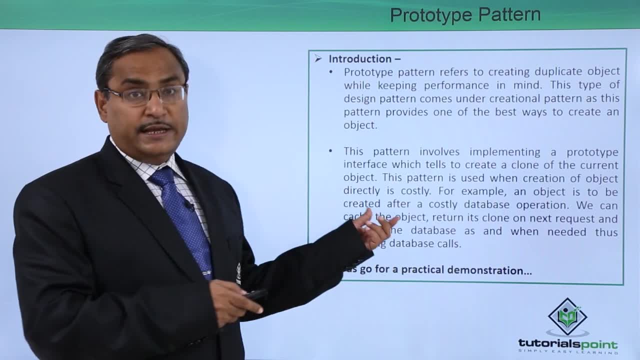 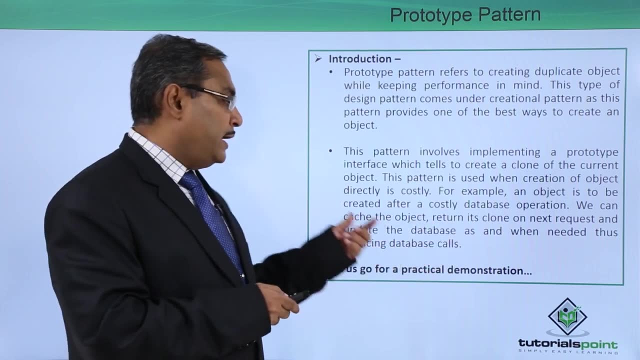 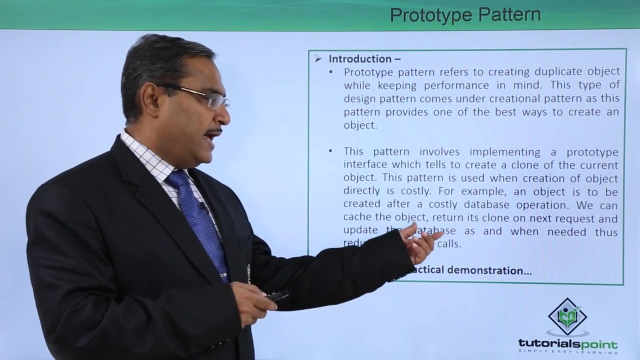 pattern is used when creation of object directly is costly. So, for example, an object is to be created After a costly database operation, we can cache the object and return its clone on the next request and update the database as and when needed, thus reducing the database calls. 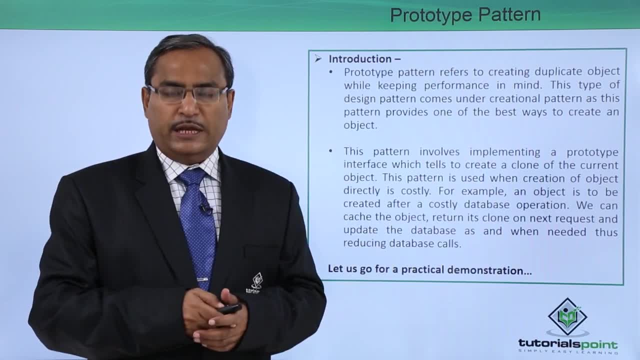 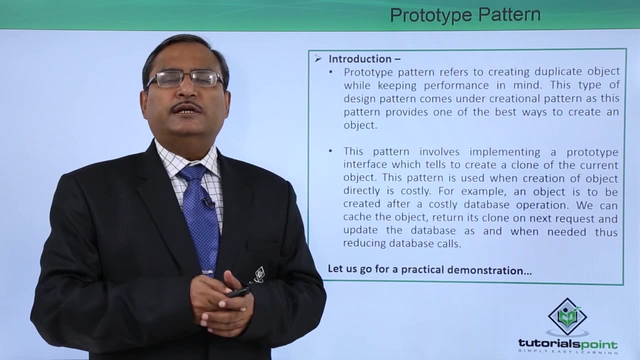 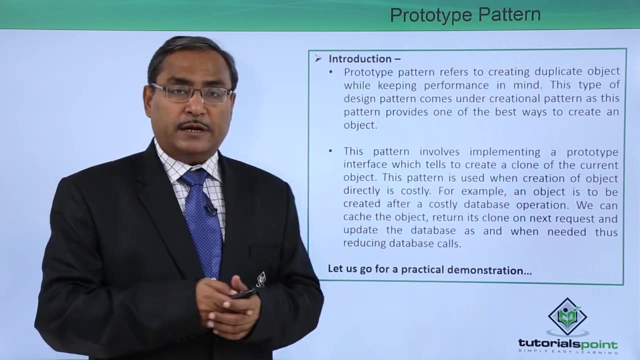 So in these applications this prototype design pattern can be used. So let us go for one practical example, using a Java application and with the respective UML class diagram. that is, a class diagram will be considering here. So here is the demonstration for you. 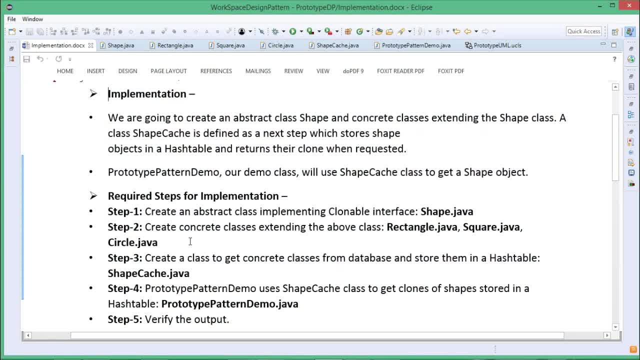 Let us discuss some Java codes to describe how this prototype design pattern can get implemented. So here we are going to create one abstract class. the name of the class will be shape and concrete classes. extending this abstract class, that is the shape, And the class shape cache is defined as the next step, which stores different types of shapes. 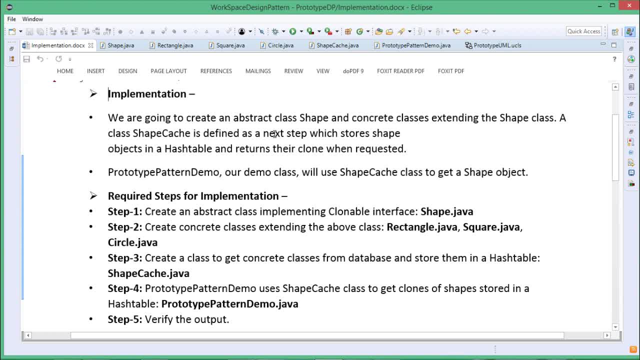 in one hash table and returns their clone when they will be requested. So prototype pattern demo will be our demo class and where we will be having our main function and we will use the shape cache class to get a shape object, passing the respective key value, and then the respective shape object will be obtained. 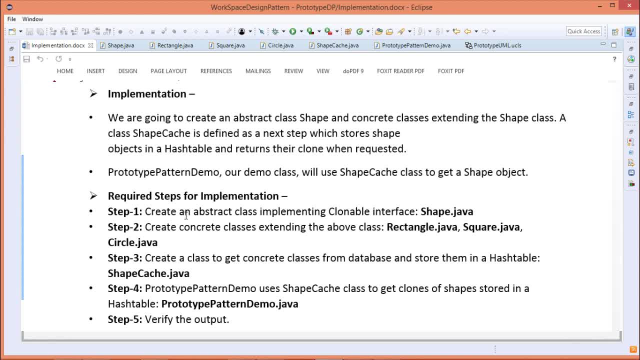 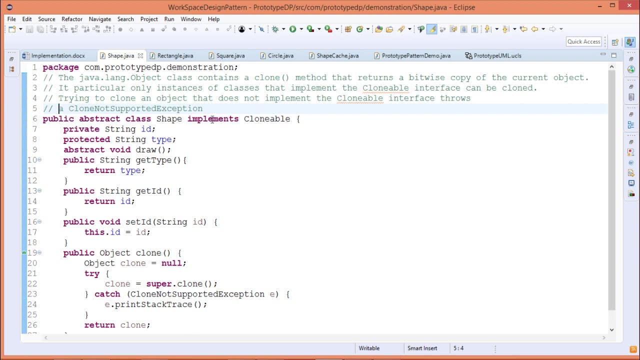 So to do this implementation, we are going through some steps. Step one: create an abstract class implementing clonable interface, and the name of the class will be shapejava. So let us go for that. So this is our shapejava, and here you see: public abstract class- shape implements clonable. 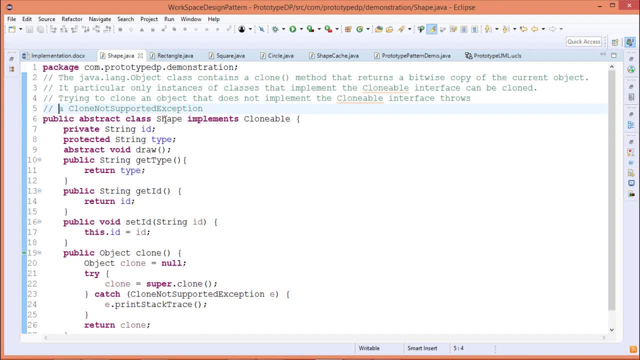 So this particular class is abstract. type name of the class is shape and implements clonable. The javalangobject class contains a method that is a clone method that returns a bitwise copy of the current object. It particular only instances of classes that implement clonable interface. 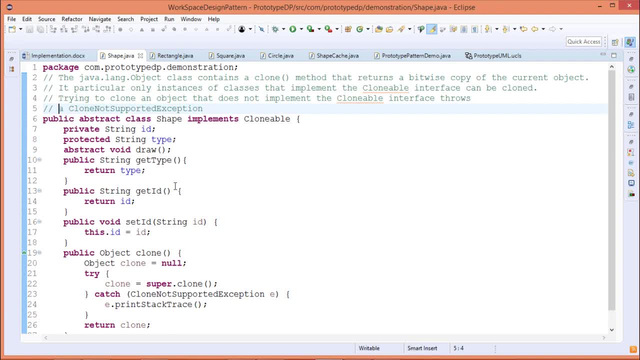 So let us go for that. So let us go for that. So it can only be cloned. So this bitwise copy of the current object can be obtained through this clone method if the class implements that cloenable interface, trying to clone an object that does not implement. 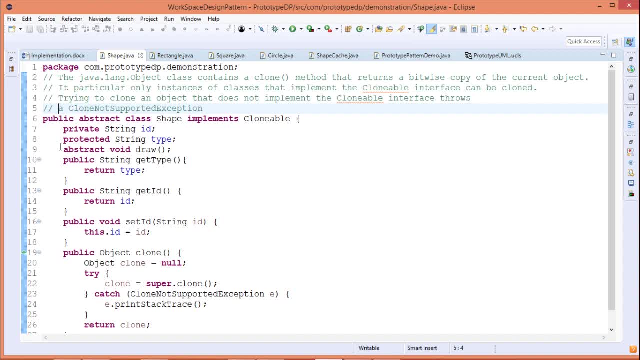 the clonable interface throws one exception and the exception name is clone- not supported exception. So if I want to use the method clone onto a particular class object which is not implementing clonable interface, then clone- not supported exception will be thrown. so here we are having. 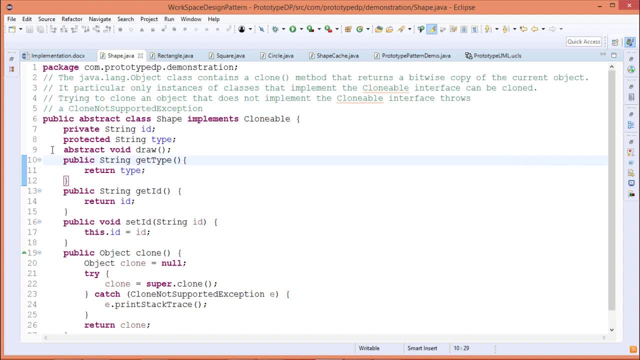 this public abstract class shape implements clonable. we're having the member variables, like your string id, string type. we're having one abstract method. there is a draw and that's why the class is also abstract. we're having one method. there is a get type which returns the type. we're 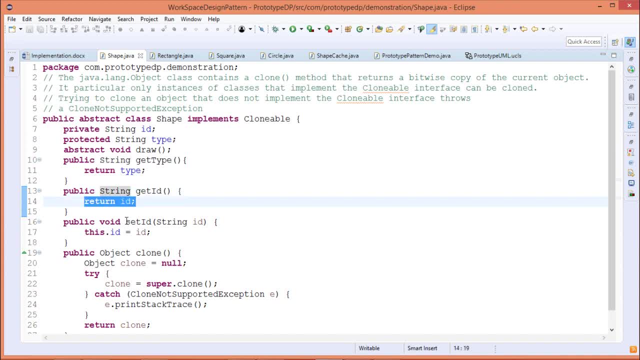 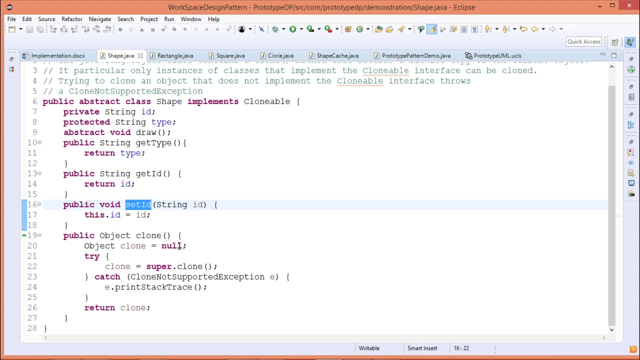 having the get id, which returns the id, and we're having the set id, where one string object will be passed as input parameter and that will initialize the id here. so this id will get initialized by the method set id. we're having one object called the clone, so object clone is equal to null. 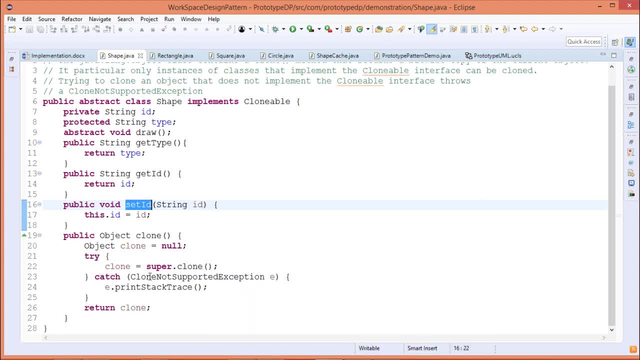 clone is equal to support dot clone and catch clone, not supported exception. so if the class does not implement this clonable interface, then this exception will be thrown. so we're having the get id which returns the id, and we're having the set id will be caught here and then it returns the clone. so there is a public object clone here. 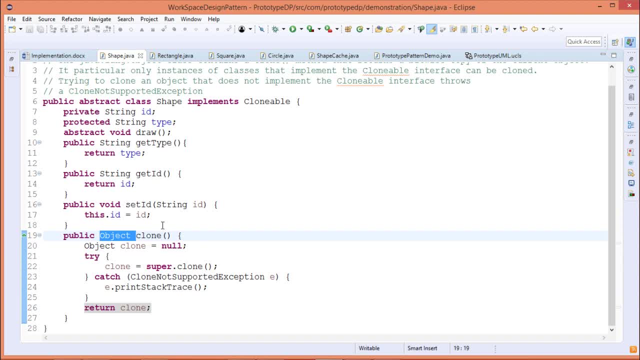 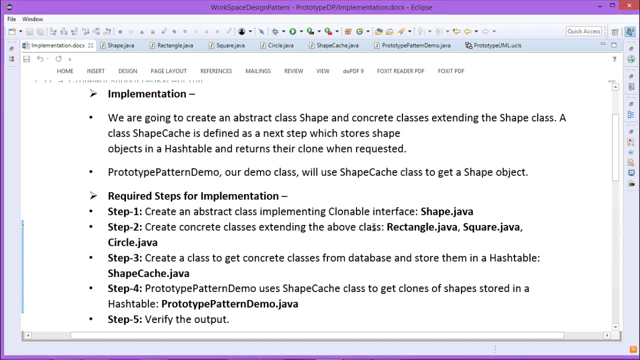 so this is the respective object which will be returned by this clone method. this clone method is there under this clonable interface. so now let us go for its next step. so let us go for the step number two: create concrete classes extending the above class, that is, the shape dot, java and the 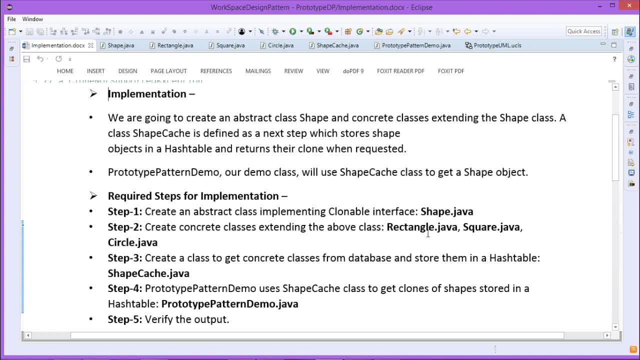 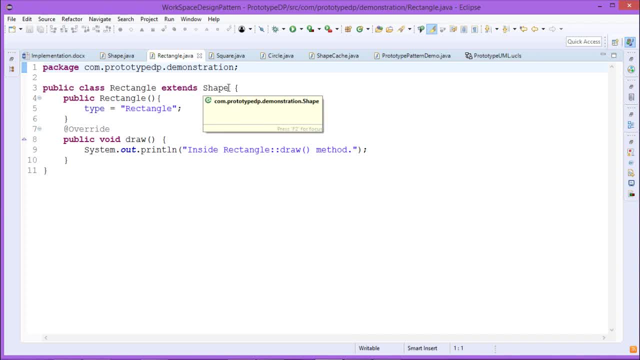 concrete classes will have the name, that is, the rectangle dot java, square dot java and circle dot java. so here we are having the rectangle dot java, which implements, which extends the shape abstract class, and here you see this. so shape is nothing but one abstract class which is containing 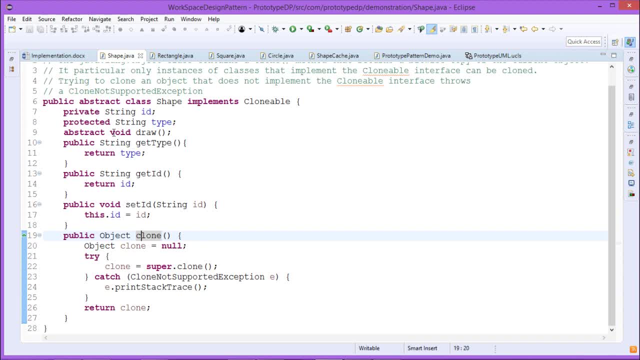 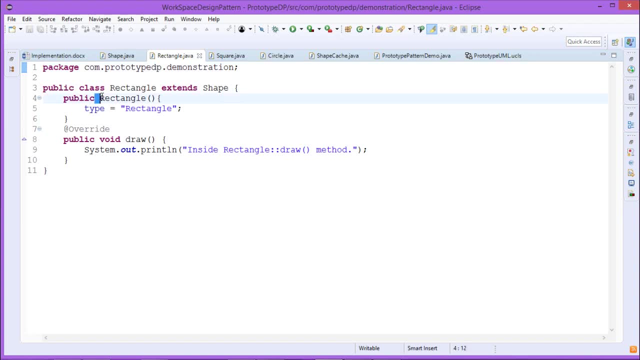 one abstract method. the name of this method is our draw. so there is a abstract method, draw here, which returns void. so this rectangle- so it is the constructor type- is equal to rectangle. so i'm initializing this type with the string rectangle and it is overwriting the method. 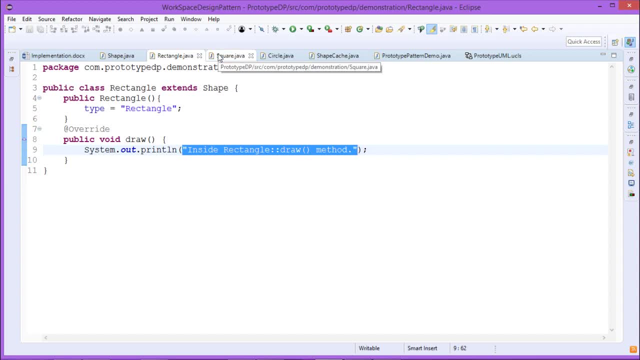 or draw, and it is printing this respective string. similarly, we have defined the another class, that is, the square, which extends the abstract class shape, and this is the respective code in front of you. we are defining another class, that is, the circle, which is extending the abstract class shape. 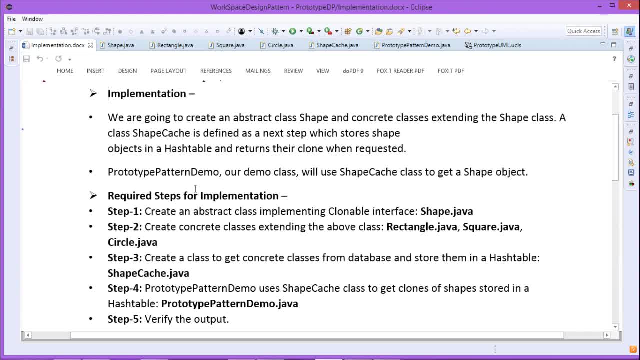 and the code is in front of you. so now let us go for create a class, to create concrete classes from database and store them in a hash table. we know that in case of hash table, it is containing key value pair, so key values will be unique and against each and every. 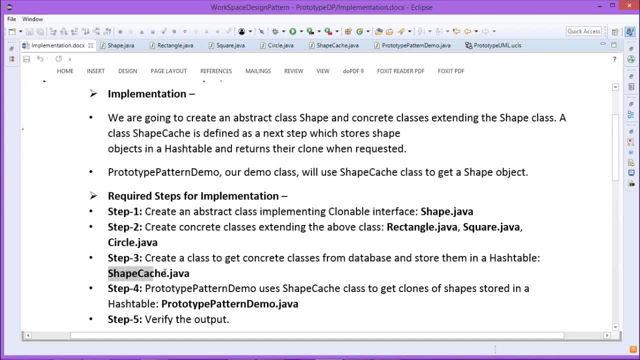 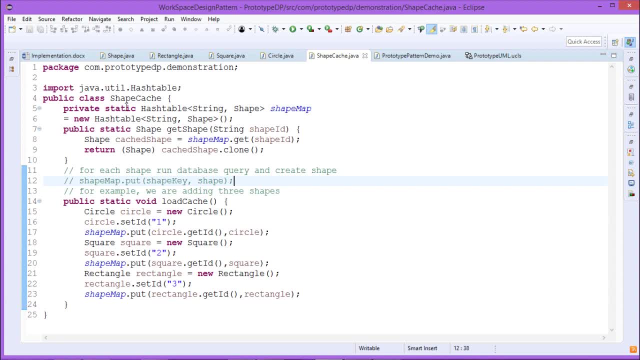 key, one value will be associated and the name of the class will be shape cache dot java. so we are going for this shape cache dot java. so here you can find. so here we are having one hash table object, that is the shape map, and it is having two things. so the first key will be of the type of 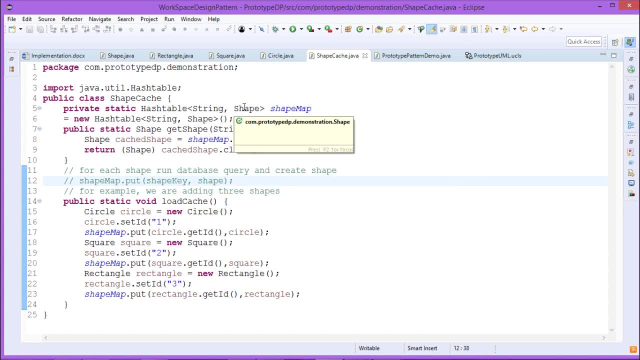 string and the second one will be the value will be of the type of shape class object. so this is the respective constructor. we have called to instantiate this shape map. so that is now. we are having the method, that is, the get shape. we are having the method called the load cache, in case. 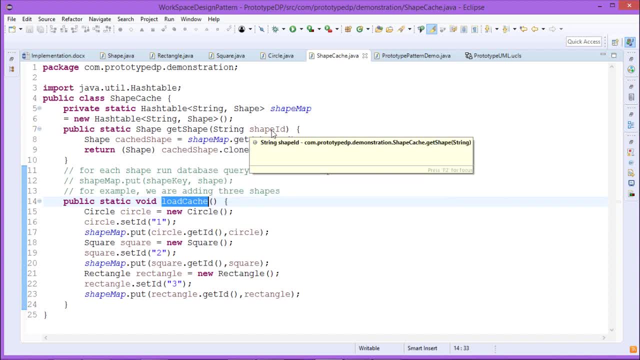 of get shape. we are taking the string that is the shape ideas input argument and then from this shape map that is the hash table. this is the hash table object here, which is from the get method. using the get method, passing this shape ideas input argument, i am getting this shape object. 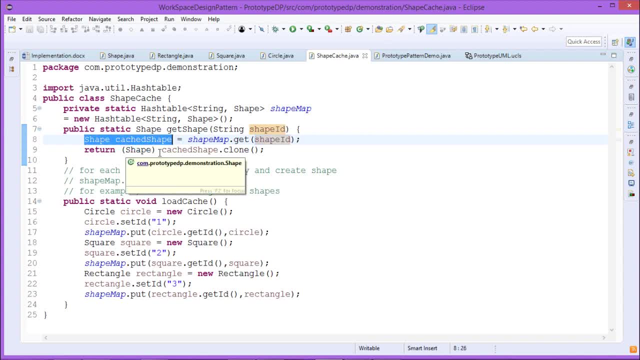 as a return and shape will be returned. at the end there is a cached shape dot clone, so the respective bitwise copy of that object will be returned and we are doing the typecasting as shape because this particular method, get shape, returns the shape class object. okay, so now this shape is nothing. 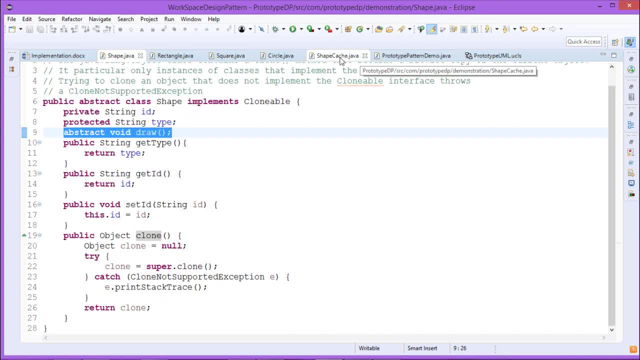 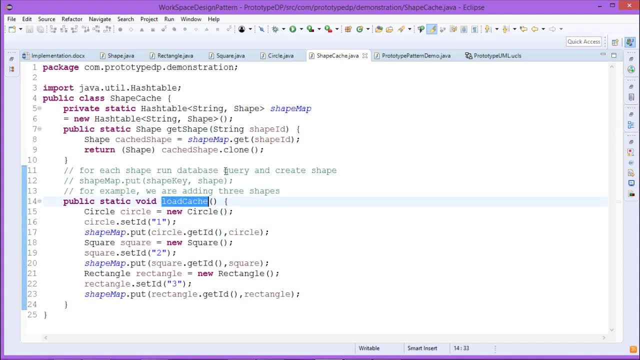 but one abstract class. we define that one earlier also. okay. next we are going for the next method. there is a load cache. so for each shape, run database query and create shape. there is a shape map dot. put shape key comma. we are having the respective shape object. for example, we can: 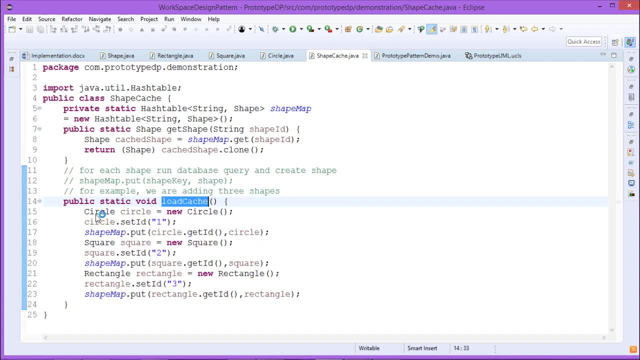 adding three shapes here, so load cache we are having. so circle circle is equal to new circle. so we are defining one circle class object and circle dot set id is equal to one. we are making making these ideas. one shape, map dot put here we are having this circle dot get id, so that is our. 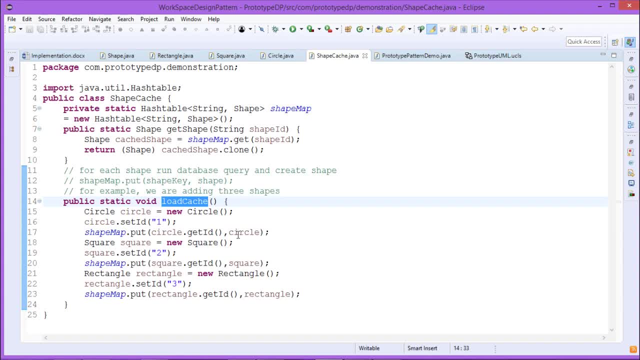 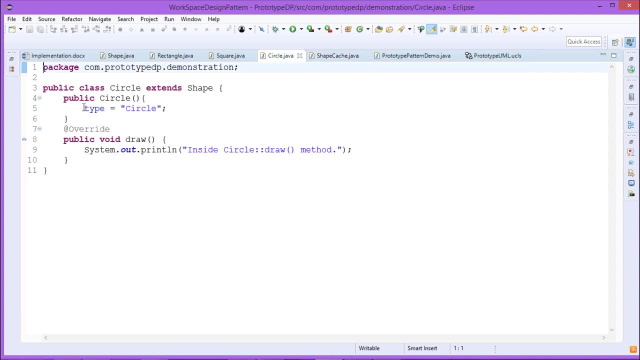 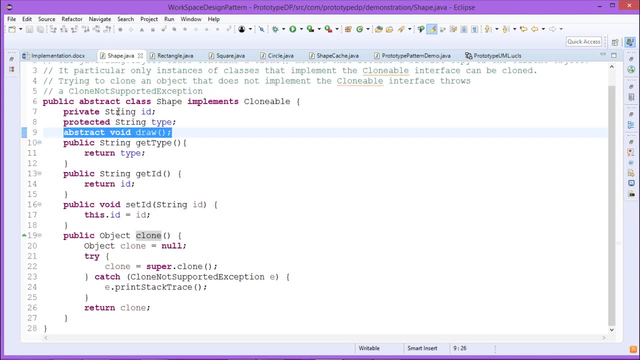 one here. and then we are passing this circle object as a second argument to this put method, so we can easily go to the circle. you can find that here it is the type is equal to circle and it is having the draw method which is implementing this abstract class shape here. so the shape is having the string. 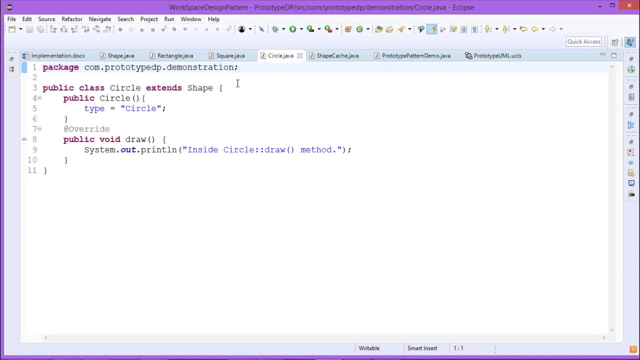 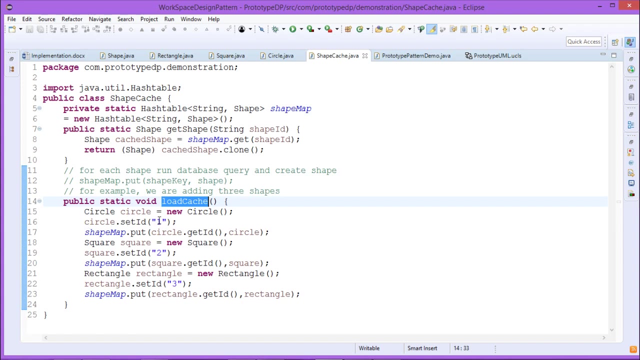 id. so that's why, whenever we are defining this, this circle class, which is extending shape, so as a result of that, this id is also becoming available from the circle class here. so that's why we are writing this one as circle dot set id1. so this one will be assigned to the id, because the code was: 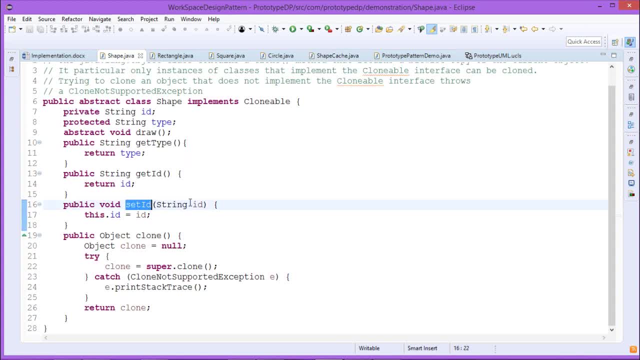 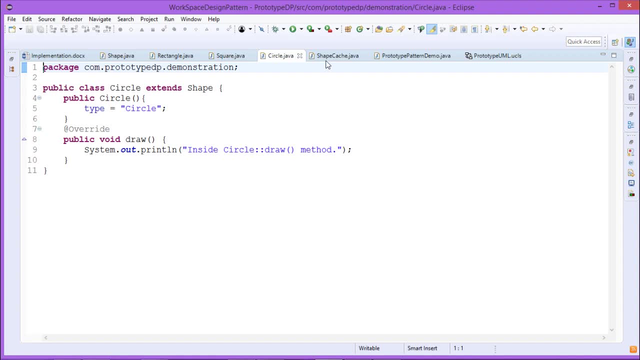 written in the shape, because we are having this shape id. so whatever the value will be passed and that will be assigned to this. that is the instance variable, that is the id here. so that method we have used here in case of shape cache. similarly, we are defining one square object. 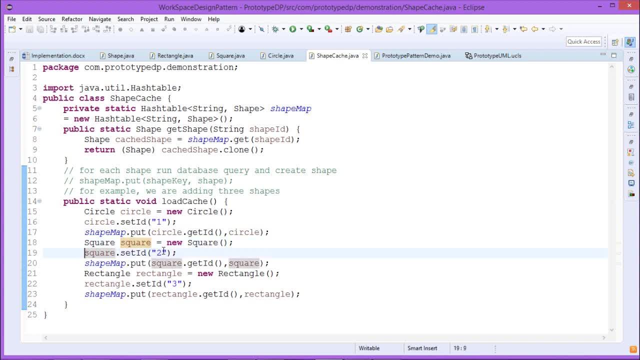 square class object. and there we are making this square dot set id 2 and then shape map dot put. we are passing this one as square dot get id and we are having this square, this object, we are writing: so this is the id, there is a key and the value paired. similarly, we are keeping this, we are keeping this rectangle. 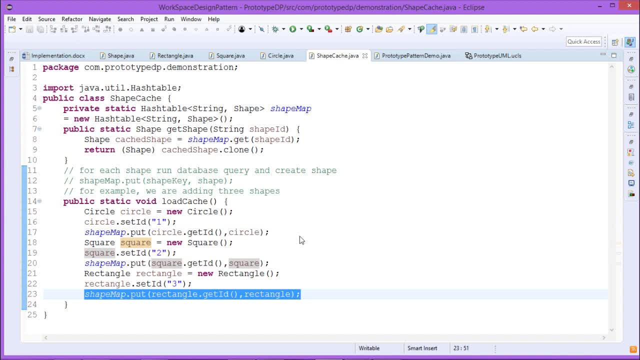 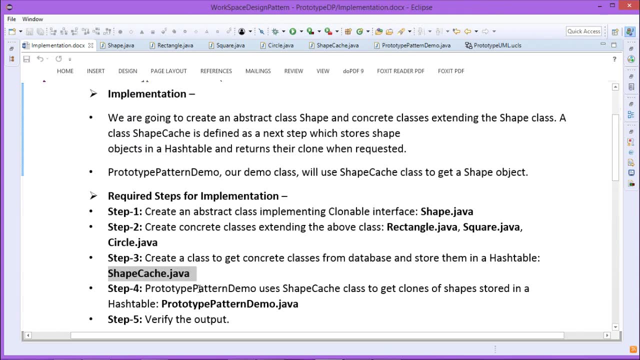 object in the respective uh hash table. object: that is a shape shape map. so now we are going for the last one. so there is a step number four. prototype pattern demo uses shape cache class to get clones of shape stored in a hash table. that is a prototype pattern demo. dot java here. so now 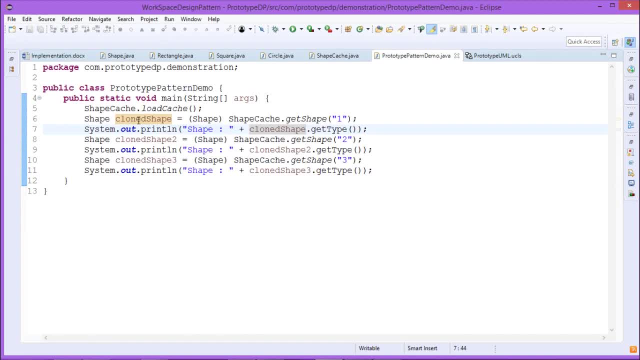 we are going for this prototype pattern, demojava. so here we are doing this one. there is a shape cache dot load cache. so that particular method has been called. so three class objects with the respective distinct ids will get mapped onto this hash table. object: there is a shape. 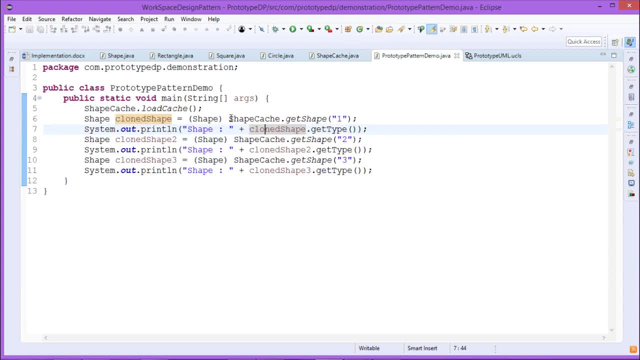 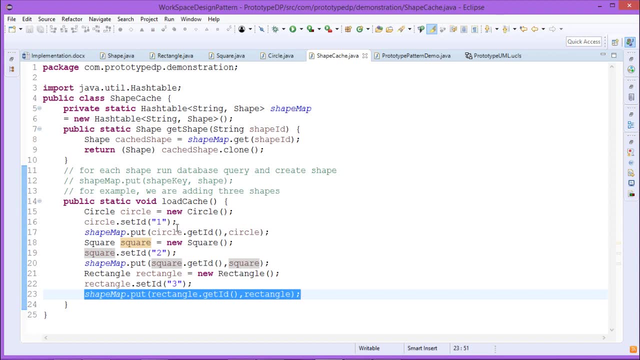 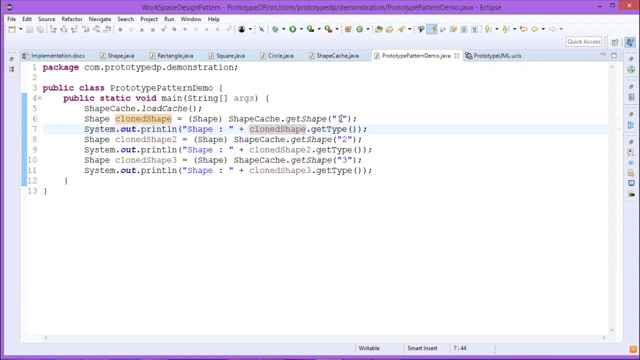 map. so now we are going for the retrieval, so we are going for this shape map dot get shape. so we are passing one. so so we are passing one. so with the one id, this circle class object was included in this shape map, was added with the shape map. so that's why this one we are passing as input. 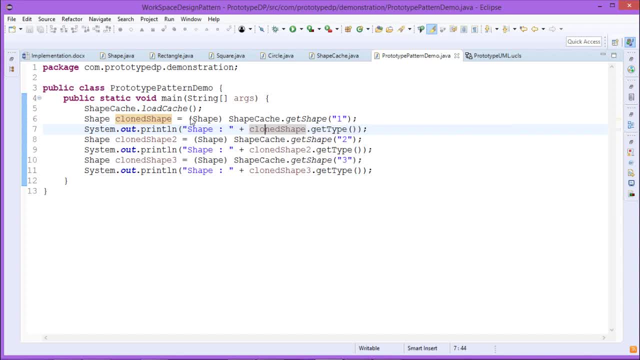 parameter. so from there it is returning the circle class object doing the type casting. so it's a shape. we are writing this one as shapecloned shape. so here we are writing the get type. so anybody writing this get type it is returning. you can easily find that in case of circle. 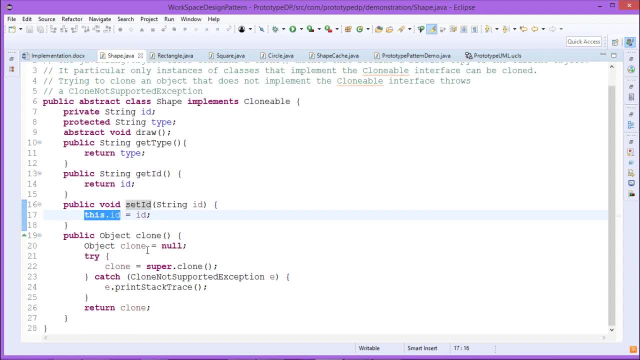 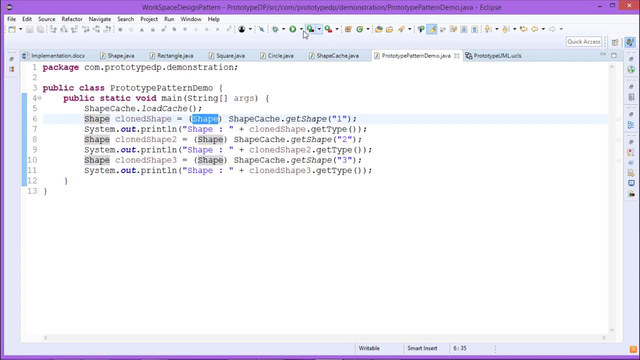 the type is assigned as circle and this get type is there, so get type is here, so it is returning the type. so that's why whenever i'm using this get type, it will print the respective string circle here, so shape colon circle. so similarly we are going for this. get shape 2: we are going for this. 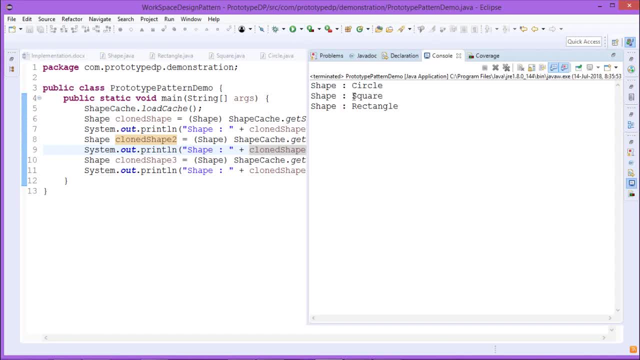 get shape 3. so in case of get shape 2, we are getting this. there is a square. in case of get shape 3, we are getting this rectangle here. so in this way, my code is uh, producing the required outputs, and from here i think you are getting this idea: how this prototype design pattern can be implemented. 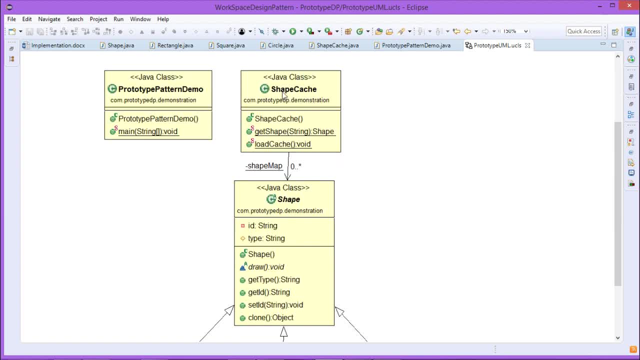 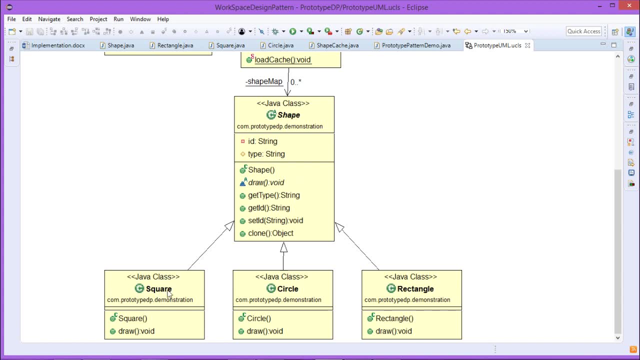 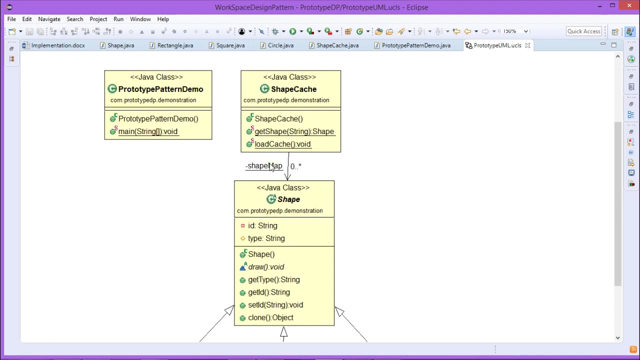 so this is the respective class diagram you are finding here. so there is a shape cache we are having. so this is a shape, is one that one of the abstract classes, so it is having the uh extended class. there is a square circle and the rectangle. the shape cache can contain all this. 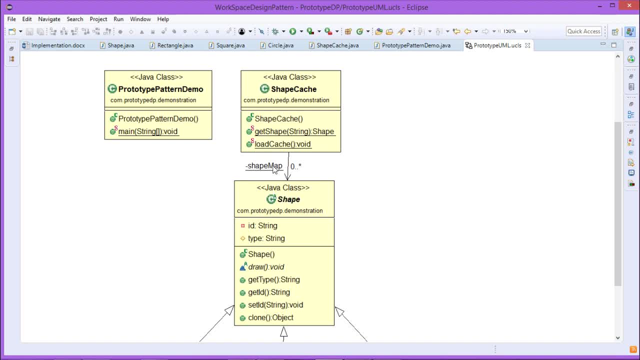 shape map objects. so shape map is nothing but one hash table object and it can contain different shape class objects and it may be ranging from zero to many. and this is the prototype pattern demo which is having the prototype pattern demo. constructor. under the public section, under the 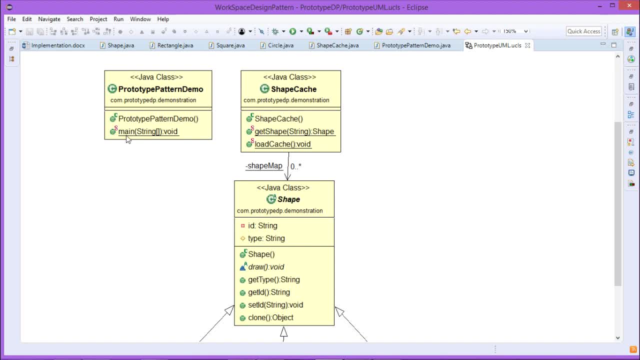 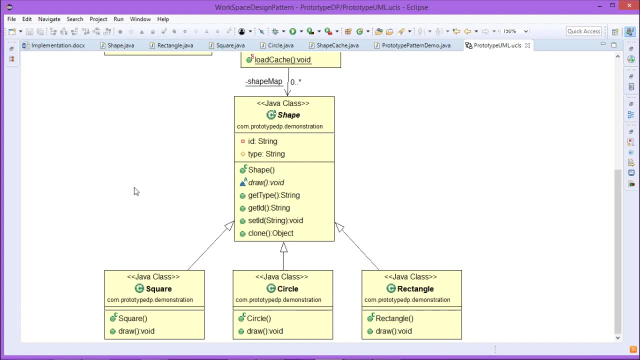 public section. we are having the method. there is a static method main here, so in this way we have shown you that how this prototype design pattern can get implemented using java. thanks for watching video.